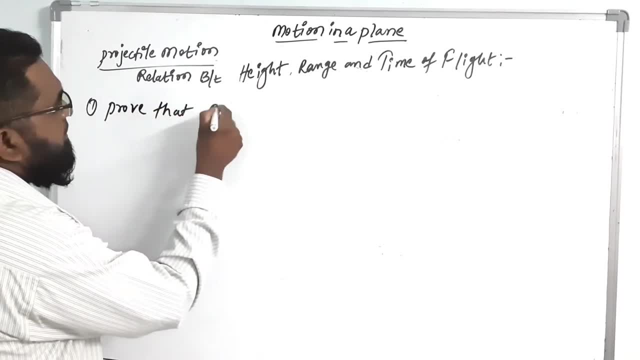 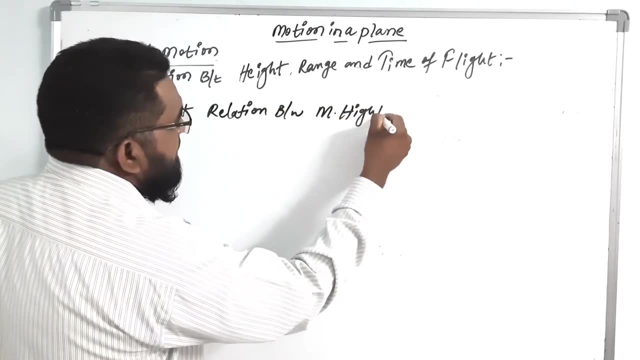 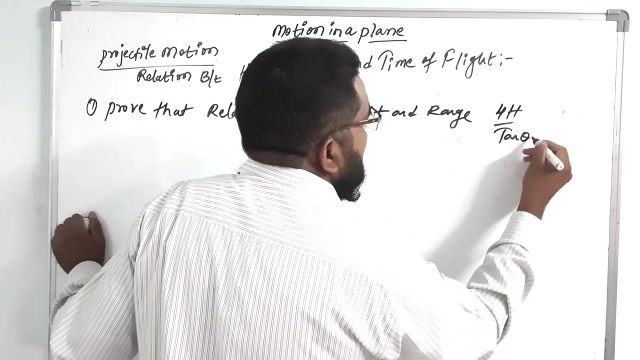 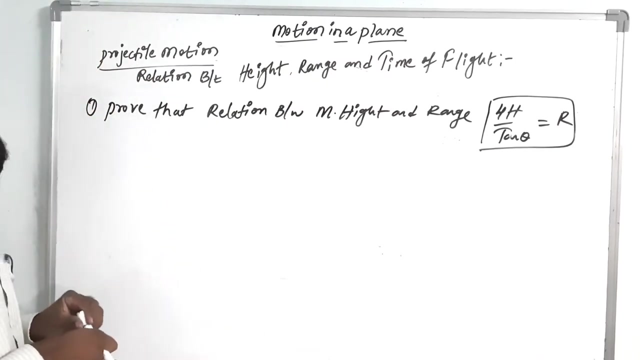 prove that. prove that relation between maximum height and range. So 4h by tan theta equal to r. Okay, first one relation: 4h by tan theta is equal to r, Proof. so what is the proof Here? 4h by tan theta is equal to r, we are proving. So first, 4 into h by tan theta. So what is the 4? 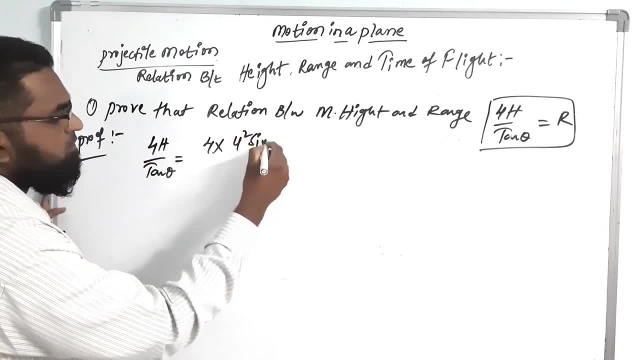 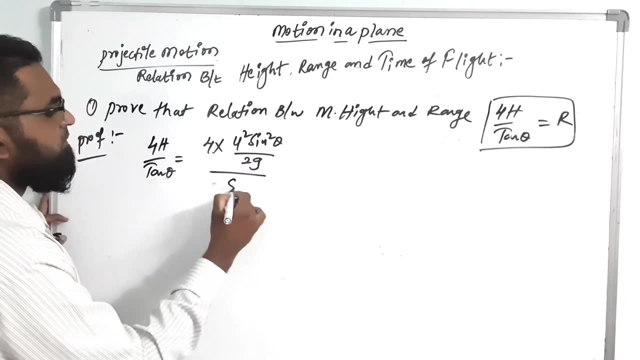 into maximum height. formula: u square sine square theta by 2g by tan theta. Tan theta means here, sine theta by cos theta, sine theta by cos theta. So okay, next to 2, 1, 2, 2 is clear. 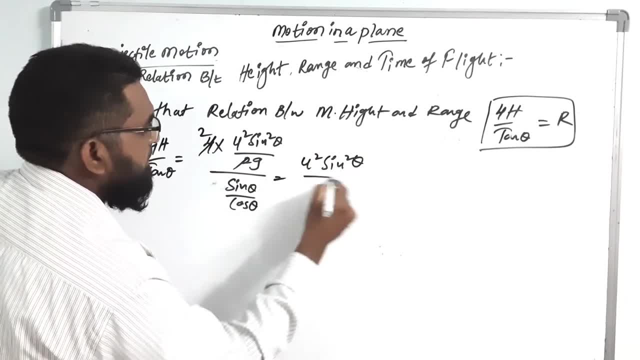 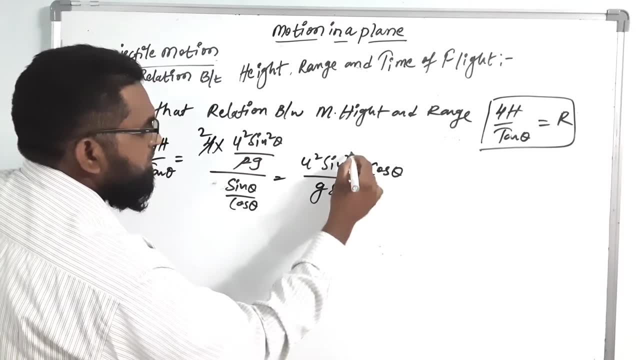 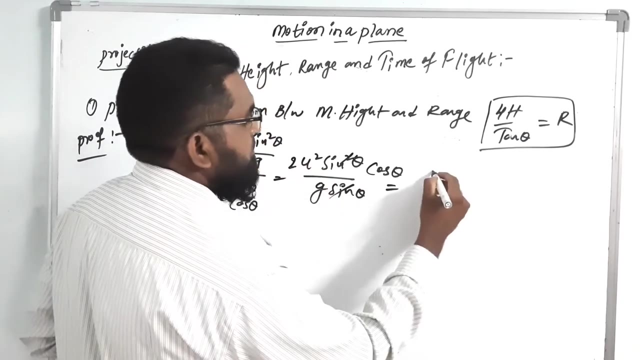 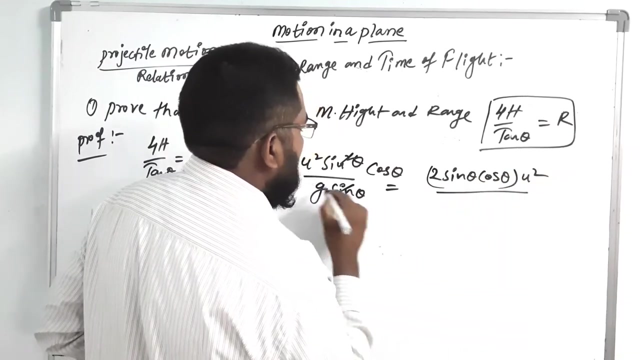 Next to u square sine square theta by into cos theta by g sine theta. So 1 sine sine cancel here. So remaining value is 2. is there 2 sine theta into cos theta into u square by u square by g, So trigonometry formula. 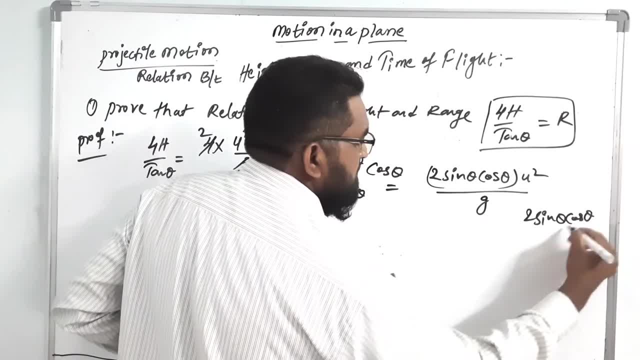 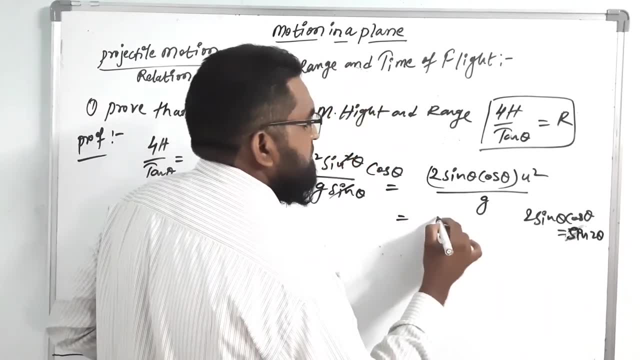 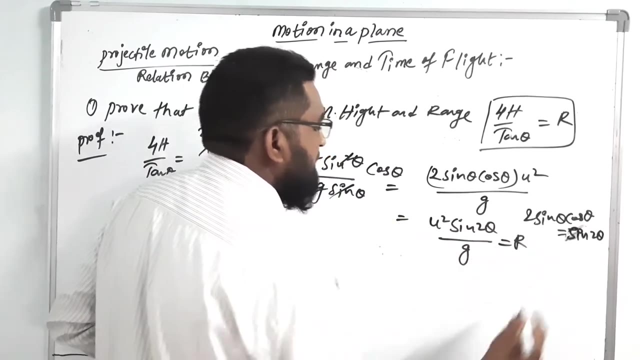 2 sine theta, cos theta is equal to 2 sine 2 theta. I hope understood this one. So u square sine 2 theta by g, So this is proved range r. So 4h by tan theta is equal to r, Proved. 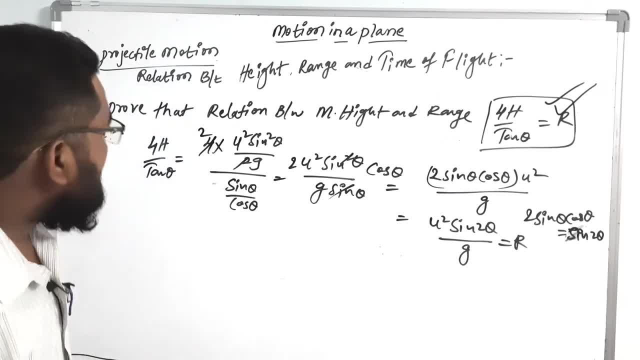 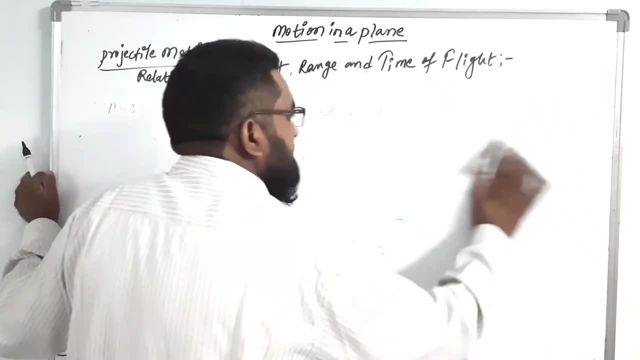 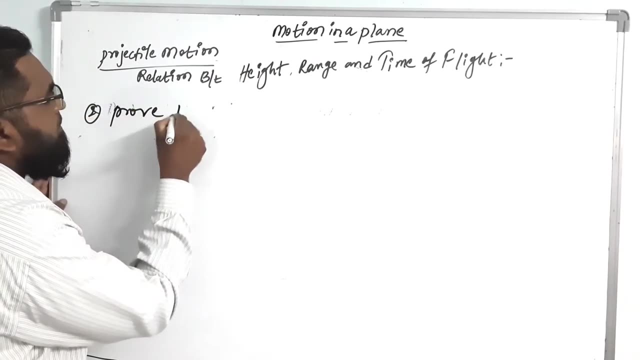 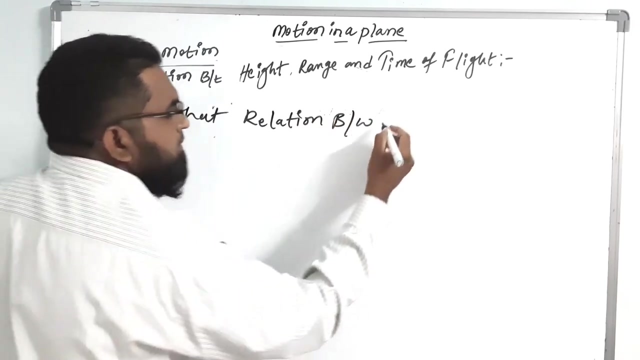 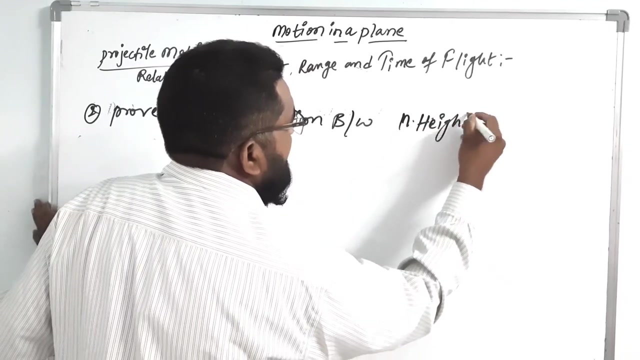 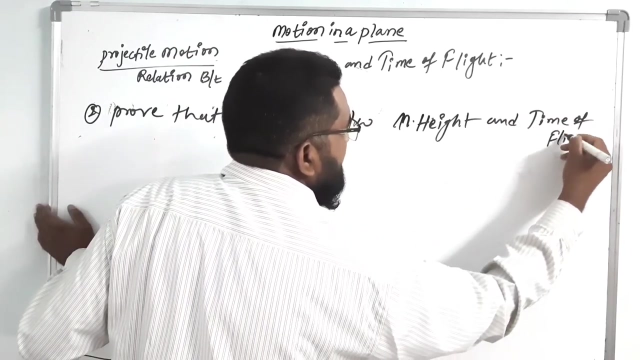 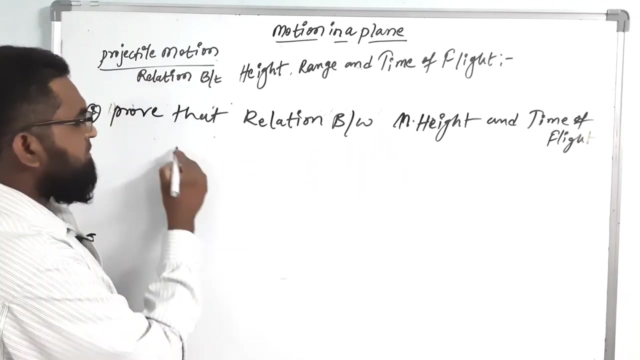 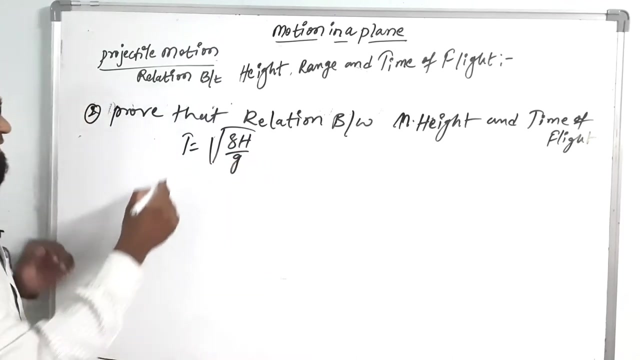 First one, this one, Next two, second one: prove that, prove that. prove that. relation between maximum height and time of flight: okay, relation between maximum height and time of flight: Okay, flight. so what is there? t is equals to root over 8 h by g. we are going to prove, prove. 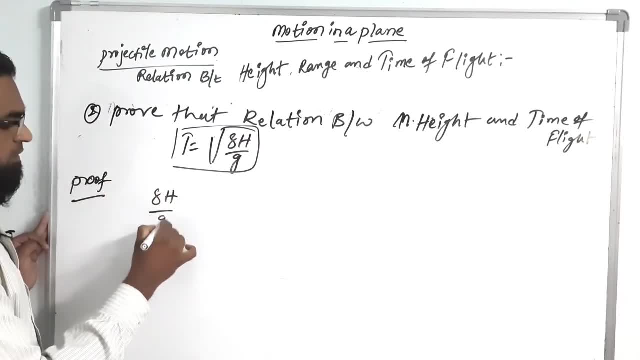 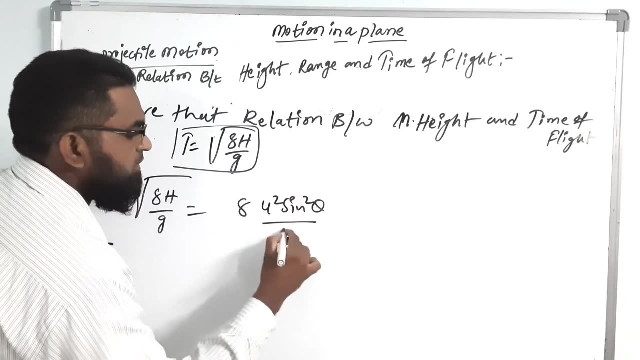 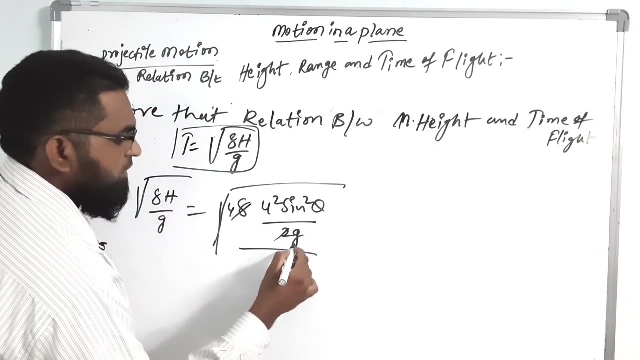 so 8 h by g, root over. so what is maximum height formula: u square, sin square, theta by 2, g by g. this is the root over 2 1s or 2, 4s, and next to here g square means finally 4 u square. 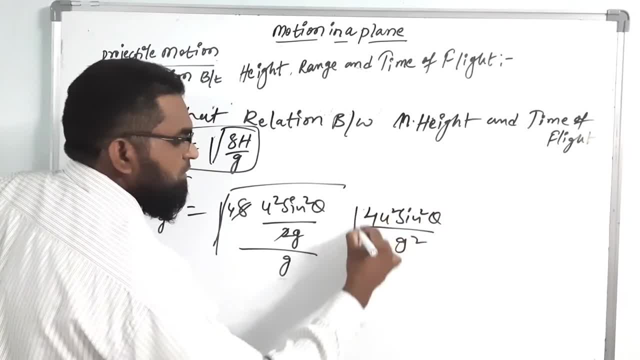 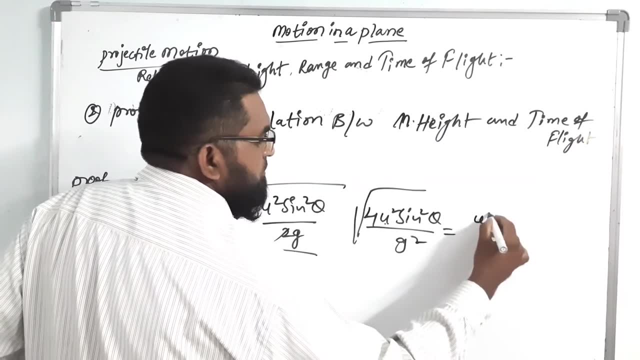 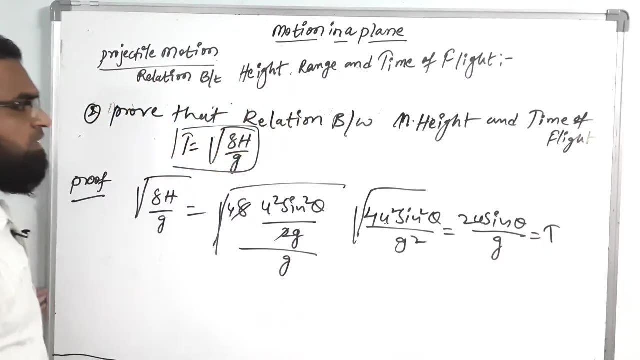 sin square theta by g square root over. so root x square x only. so 4 u square sin square theta by g. square means u sin theta by 2, u sin theta by g. so this is the time of flight. and second one also proved. next, third one: 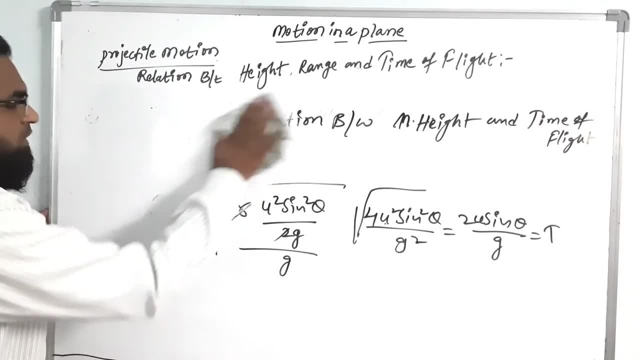 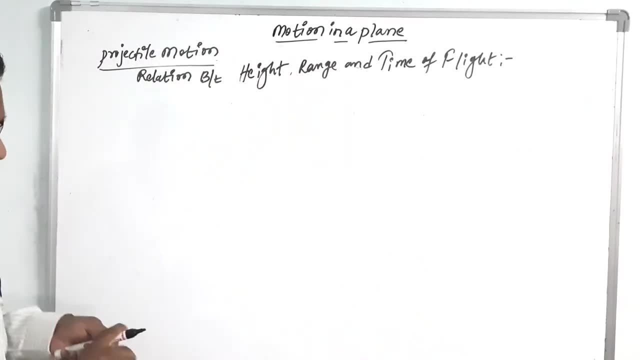 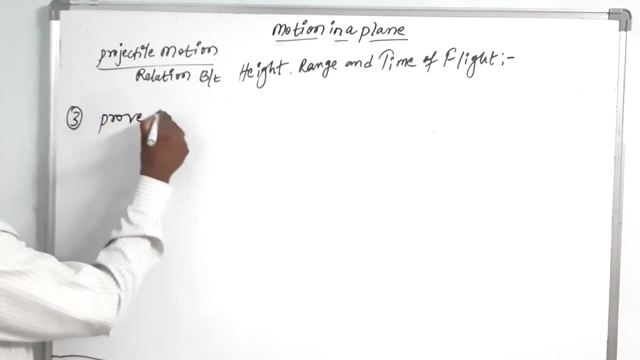 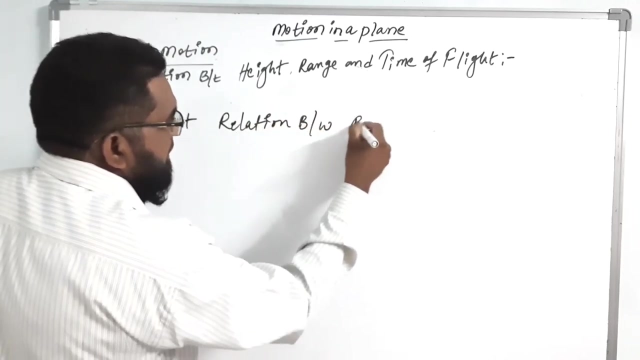 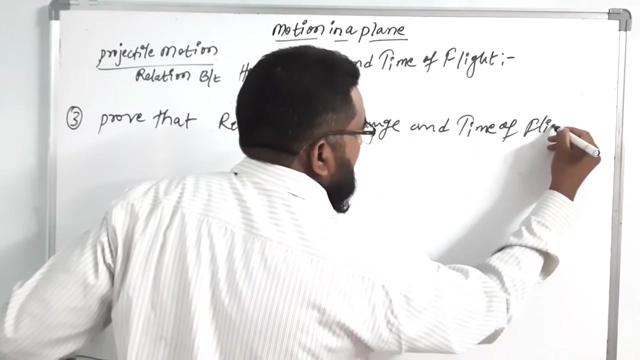 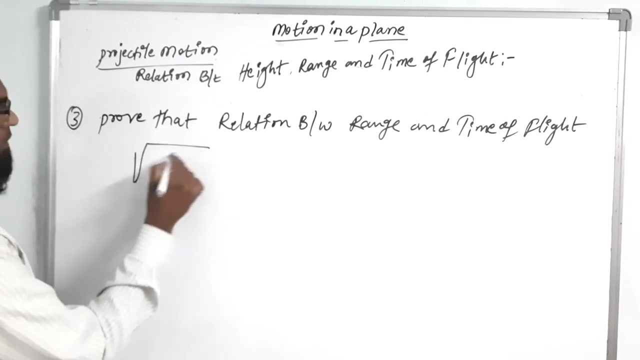 so i hope understood all things. next to next, third one: prove that relation between range and time of flight. so relation between, is given root over 2 r tan theta by g, equal to t. so we are going to prove what is there to root over 2 r sin theta by 2 r tan theta by g, equal to t. so first, what is there? 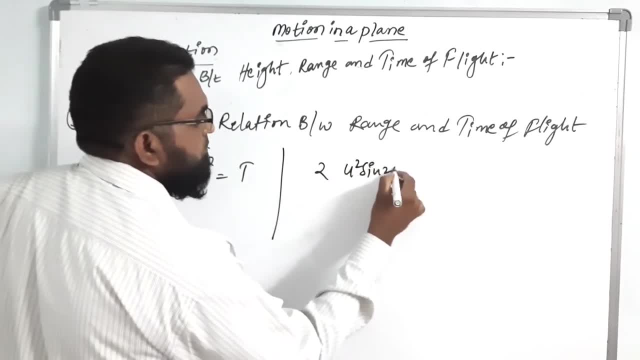 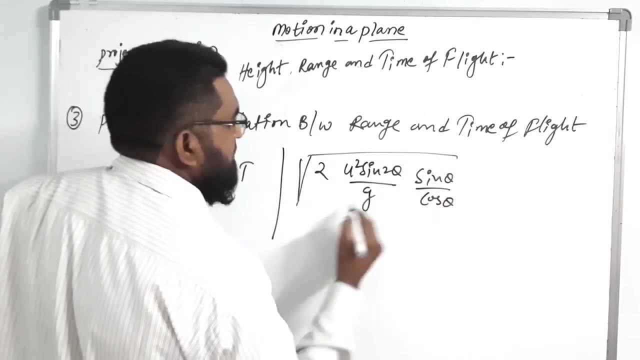 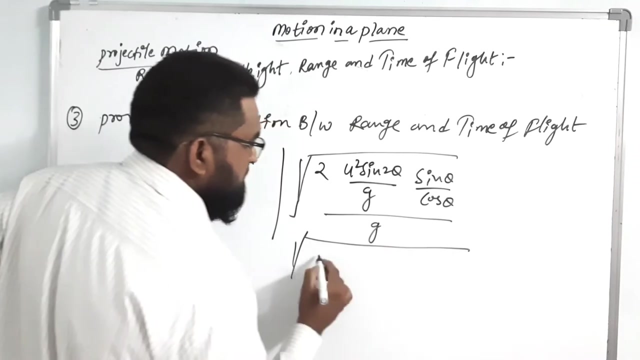 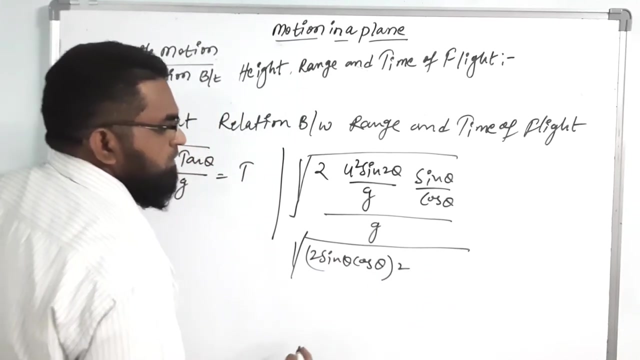 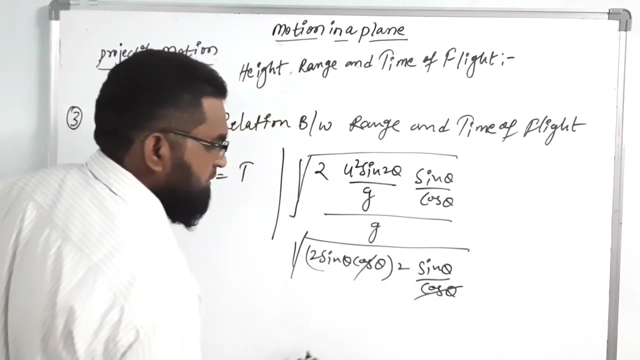 2 into u square, sin 2 theta by g, into sin theta by cos theta. root over 4. so u to V root of sin't formula. I root over g. so I know sin2 theta formula. now what's through sin2 theta form, la2 sine t cost AAA into two 2, into twice theta, into 2 x sin theta via cos theta mailing. 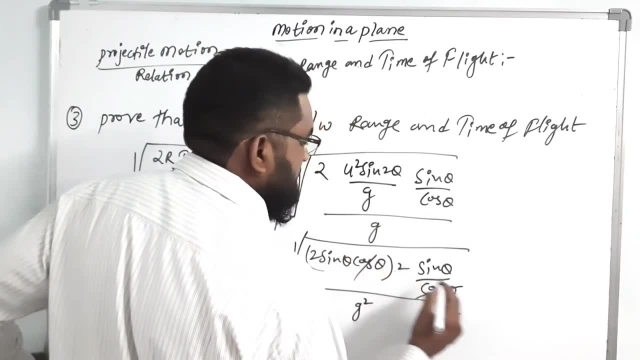 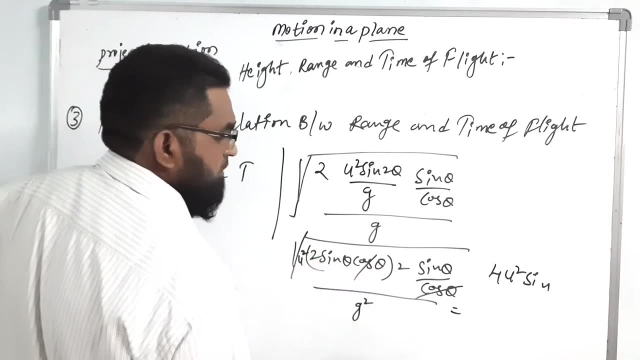 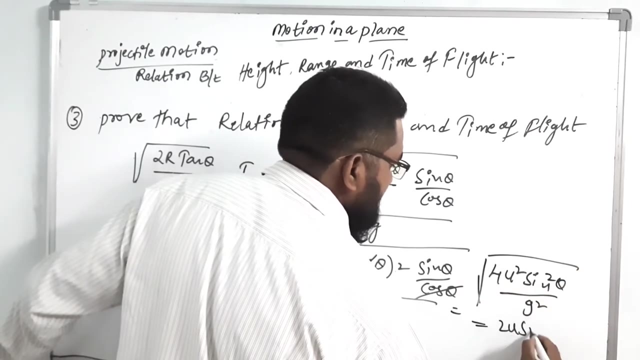 are gospel, so fire housing difficult. so finally 2 into 24. result: 4 u square, 4 u square, here u square also is there 4 u square sine square, theta by g, square root over. So finally 2 u sine theta by g. This is the relation between range and 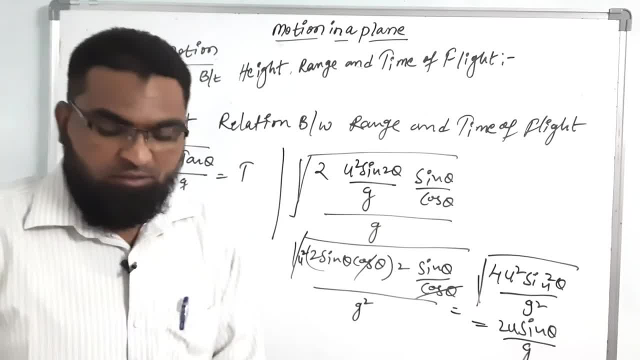 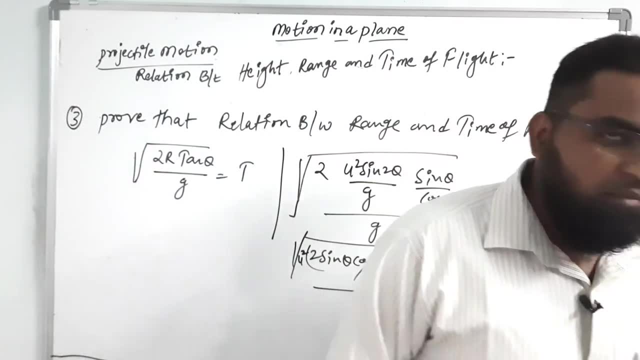 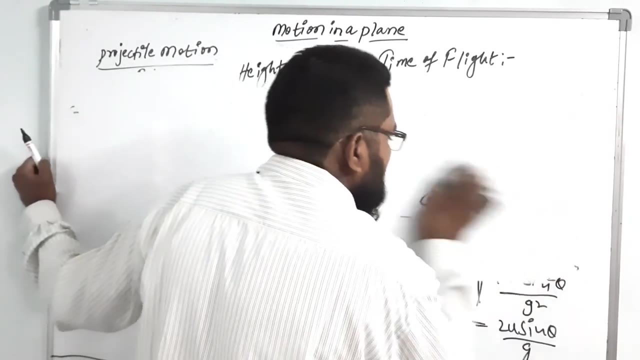 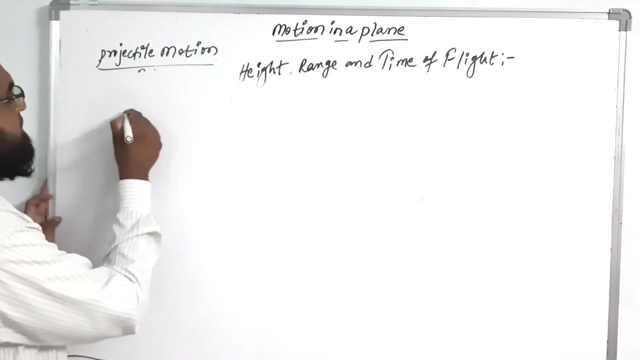 time of flight. I hope understood these three relations. So one more relation is there in projectile equation. trajectory equation in terms of are. in terms of range: see here acağım relation Relation: trajectory equation. trajectory equation in terms of DIRECT Stew. It depends upon the voting applicant area and it depends upon ヌ. 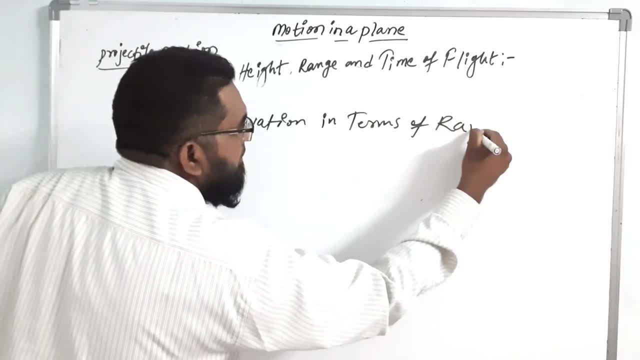 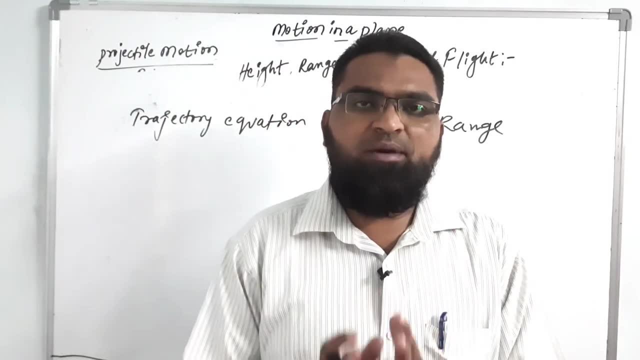 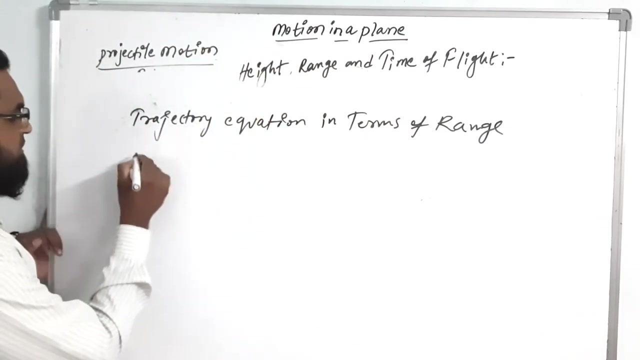 range. In terms of range means. we know already tragic equation: y is equals to x tan theta, minus half into g, into x square, by u square cos square theta. But we are using here in terms of range means, here first what is the range? r is equals to u square sin 2 theta. 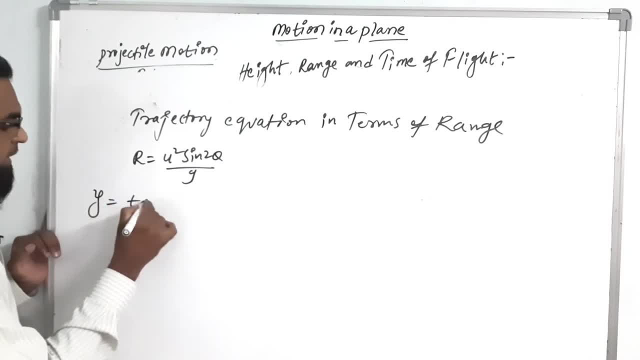 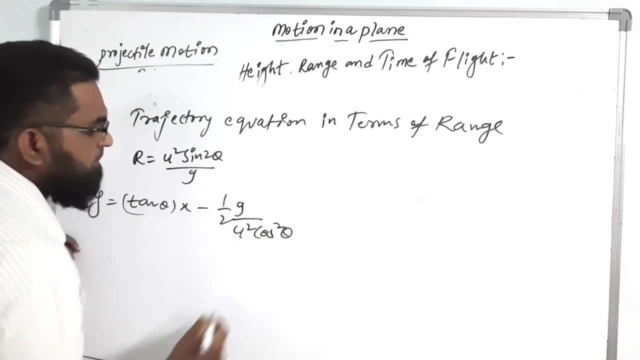 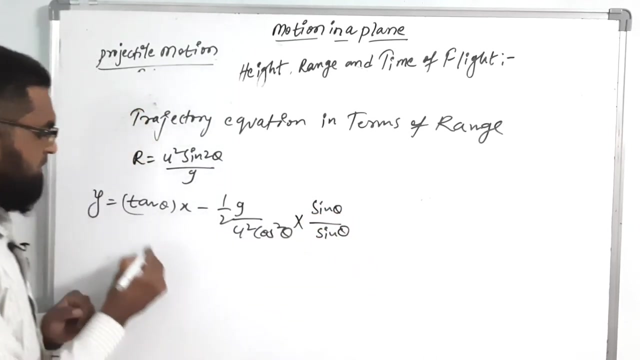 by g. So tragic equation: y is equals to tan theta into x minus half into g, into g by u square cos square theta. This equation, we are multiplying sin theta by sin theta. See what happened here. So y is equals to tan theta into x minus into g. x square is also. 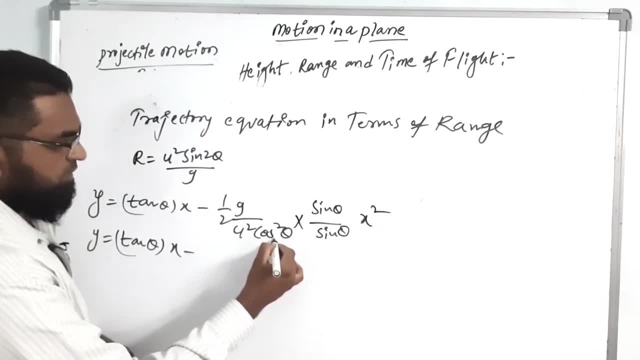 is there. So here sin theta and cos theta. 1 tat is the forming. 2 sin theta and cos theta. here, half into g into x square: 1 sin theta and cos theta tan theta. Ok, Next, 2 into 1, cos theta is there and sin theta. 2 sin theta, cos theta sin sin 2. 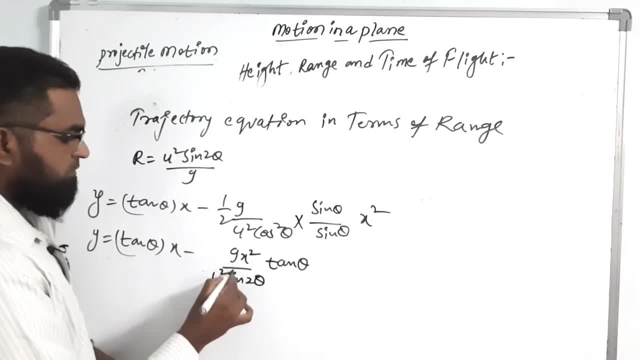 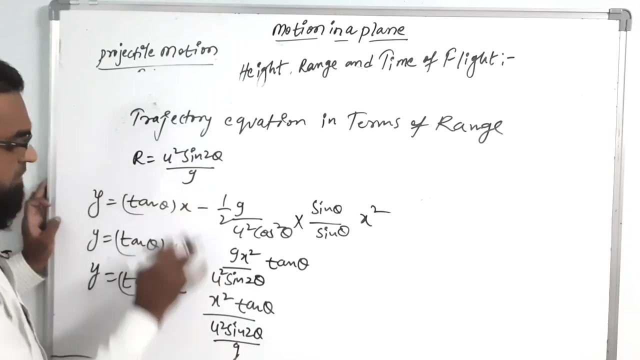 theta ok into u square. So in terms of range. so y is equals to tan theta into x minus this is: I am writing x square into tan theta by u square. sin square sin 2 theta by g. u square sin 2 theta by g. this is range formula. So multiplying here by you are substituting a.